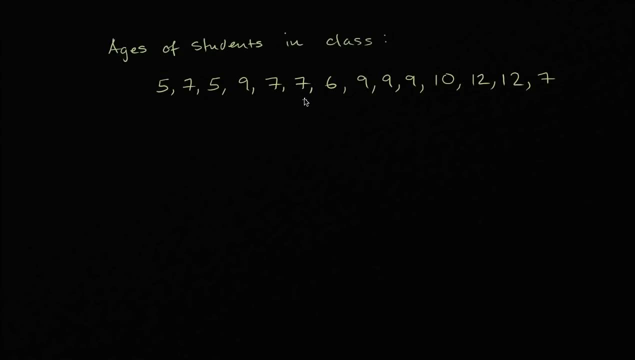 What I have here is the list of ages of the students in a class, And what I want to explore in this video is different ways of representing this data and then see if we can answer questions about the data. So the first way we can think about it, 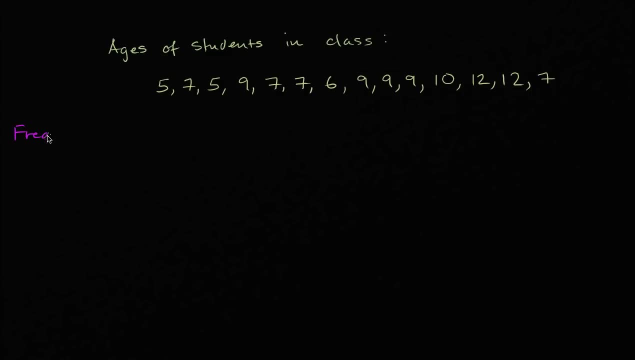 is as a frequency table, Frequency table, Frequency table, And what we're going to do is we're going to look at each for each age, for each possible age that we've measured here. See how many students in the class are of that age. 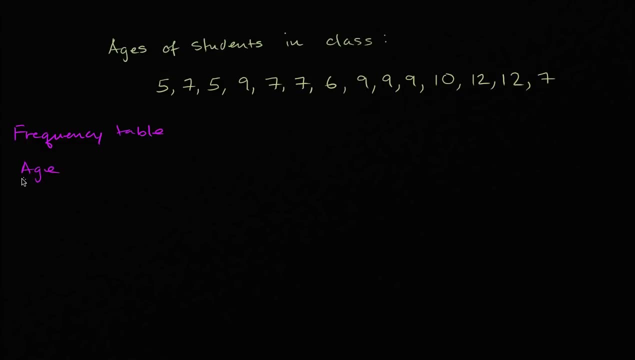 So we could say the age is one column And then the number, The number of students of that age. Or we could even say the frequency. Frequency: When people say how frequent do you do something, they're saying how often does it happen? 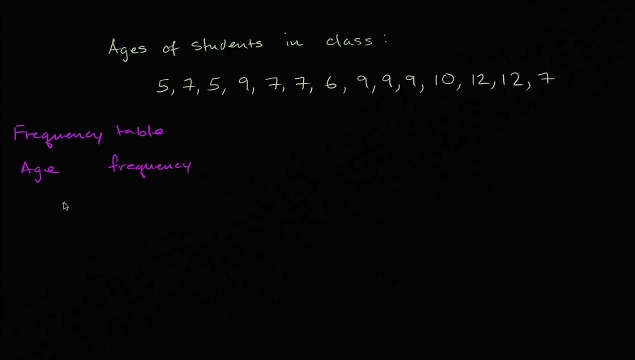 How often do you do that thing? Frequency, Or we could also say, actually, let me just write number. I'm always a fan of the simpler Number at Age, Which we could also consider the frequency at that age, Frequency of students. 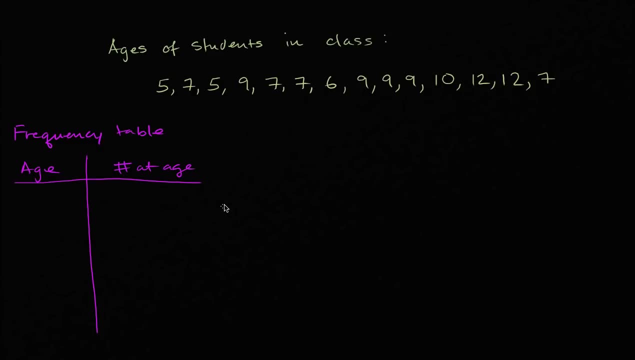 Alright. So what's the lowest age that we have here? Well, the lowest age is five, So I'll start with five. And how many students in the class are age five? How frequent is the number five? Let's see there is one, two. 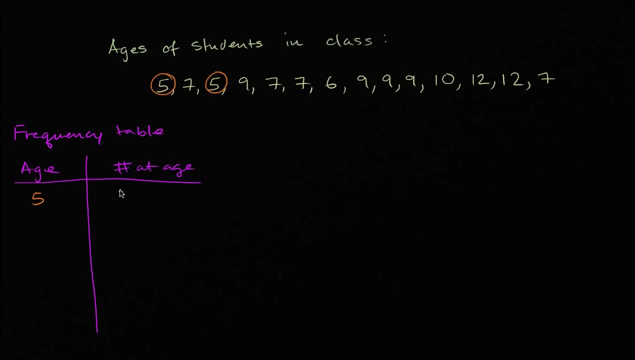 Let me keep scanning. Looks like there's only two fives, So I could write a two here. There are two fives, And now let's go to six. How many sixes are there? Let's see, there is one six. 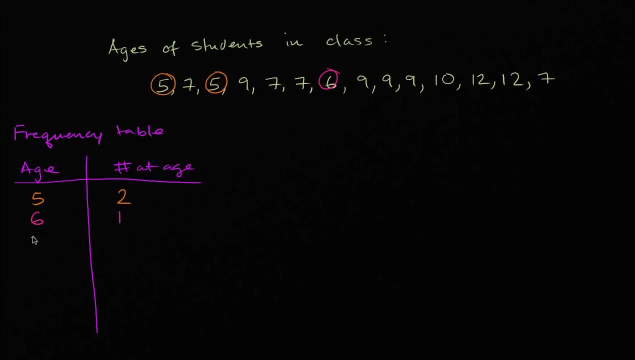 There's only one six year old in the class. Alright, seven year olds. See, there is one, two, three, four, seven year olds. Four seven year olds. Now what about eight year olds? Eight year olds? I'm gonna do this in a color. 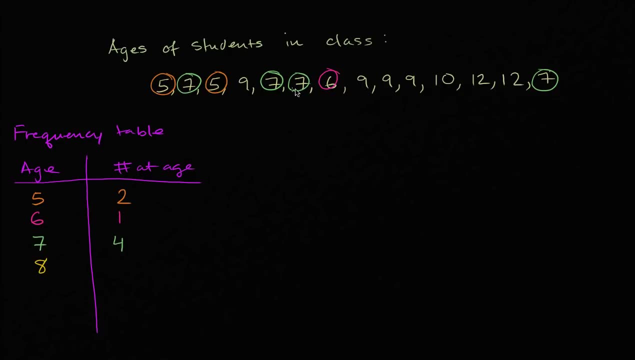 that I have not used yet. Eight year olds. we have no eight year olds, Zero eight year olds. And then we have nine year olds. Let's see nine year olds. We have one, two, three, four, nine year olds. 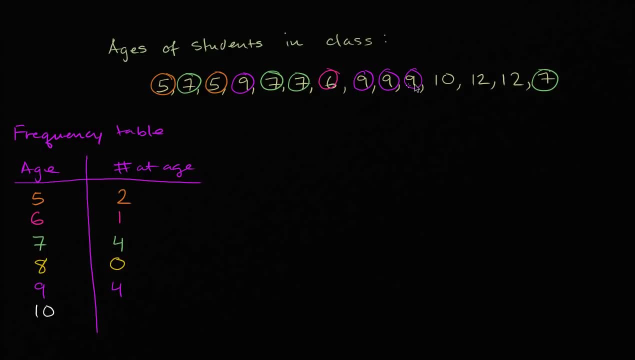 Four, nine year olds, 10 year olds. what do we have? We have one 10 year old right over there, And then 11 year olds, 11 year olds. there are no 11 year olds. And then let me scroll up a little bit. 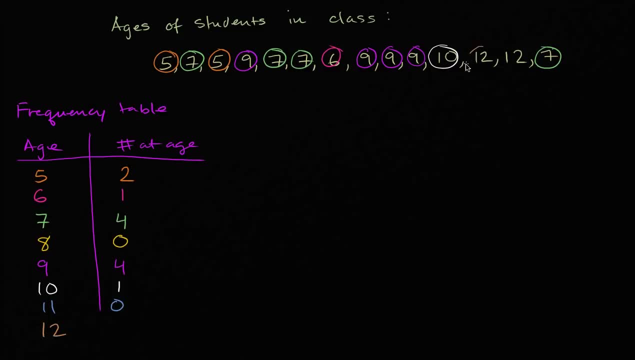 And then finally 12 year olds. 12 year olds, There are one, two 12 year olds. So what we have just constructed is a frequency table. It's a frequency table, You can see. you can see for each age how many students are at that age. 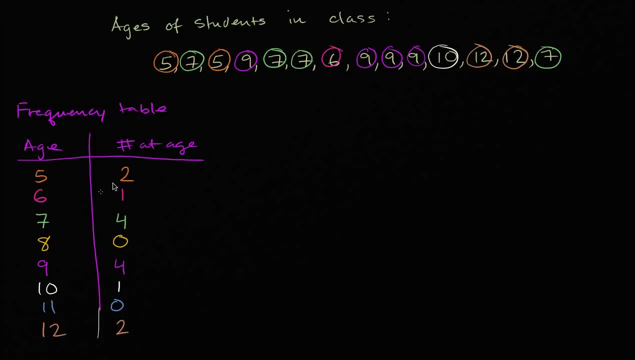 So it's giving you the same information as we have up here. You could take this table and construct what we have up here. You would just write down: two fives, one, six, four, sevens, no eights, four nines, one, 10,. 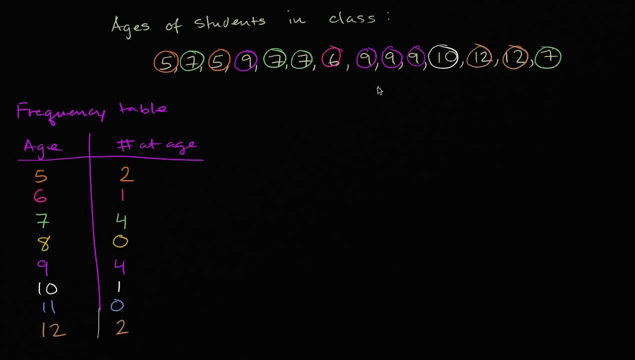 no 11s and two 12s, And then you would just have this list of numbers. Now, a way to visually look at a frequency table is a dot plot. So let me draw a dot plot right over here. So a dot plot. 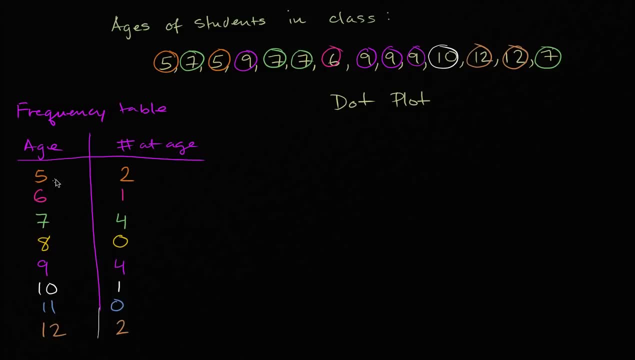 And a dot plot. we essentially just take the same information and even think about it the same way, but we just show it visually. So in a dot plot, what we would have in a dot plot, what we would have of actually, let me just not draw an even arrow there. 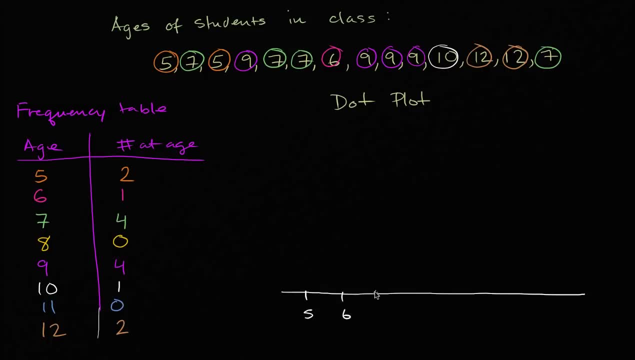 we have the different age groups, So five, six, seven, eight, nine, 10,, 11, and 12.. And we have a dot to represent, or we use a dot for each student at that age. So there's two five-year-olds, so I'll do two dots. 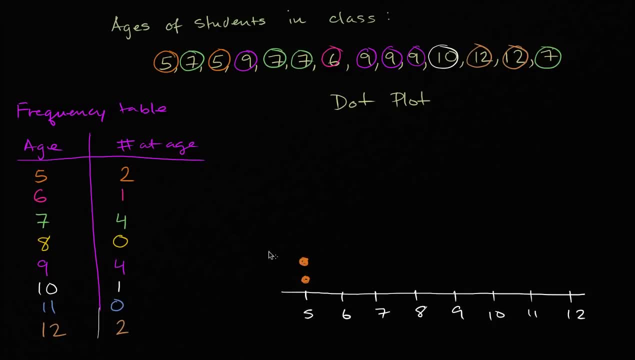 One and two. There's one six-year-old, so that's going to be one dot Right over here. There's four seven-year-olds, so one, two, three, four dots. There's no eight-year-olds, there's four nine-year-olds. 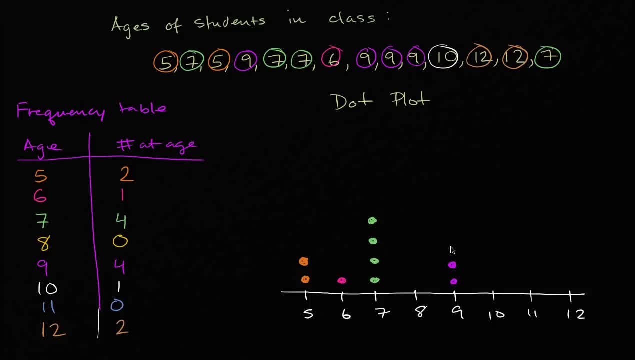 So one, two, three and four. There's one 10-year-old, so let's put a dot, one dot right over there for that one 10-year-old. There's no 11-year-old, so I'm not going to put. 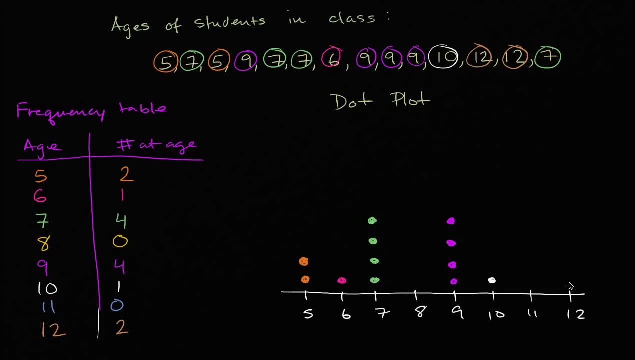 any dots there. And then there's two 12-year-olds, So one 12-year-old and another 12-year-old. so there you go. We have frequency table, dot plot, list of numbers. These are all showing the same data. 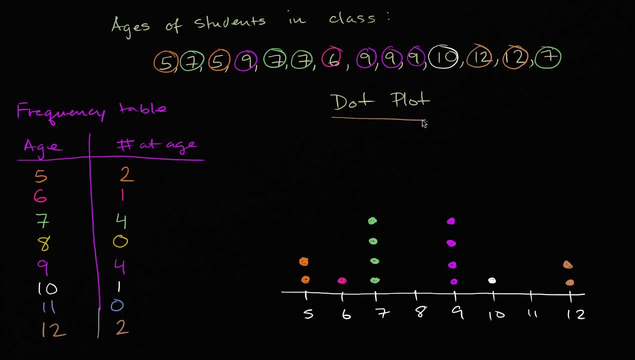 just in different ways. Once you have it represented in any of these ways, we can start to ask questions about it. So we could say: what is the most frequent age? Well, the most frequent age when you look at it visually. 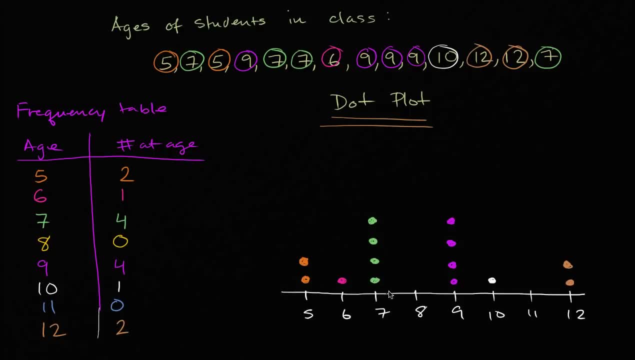 or the easiest thing might be: just look at the dot plot because you see it visually- the most frequent age are the two highest stacks, So there's actually seven and nine are tied for the most frequent age. You would have also seen it here. 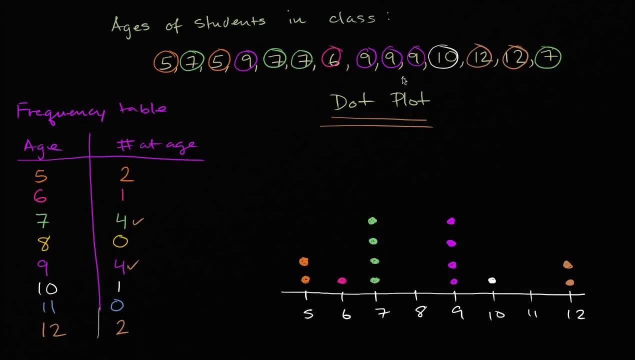 where seven and nine are tied at four. And if you just had this data, you would actually you'd have to count all of them, to kind of come up with this again and say, okay, there's four sevens, four, nines. 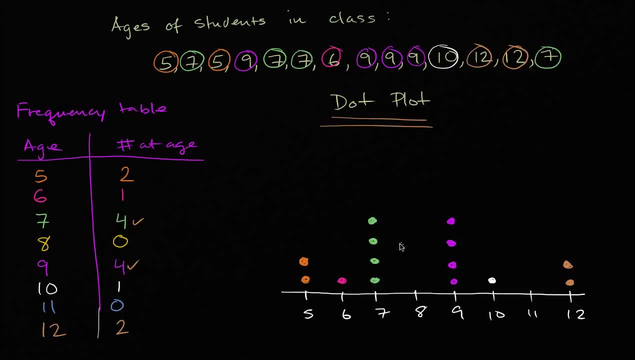 that's the largest number. So this is: if you're looking for what's the most frequent age, when you just visually inspect here it probably pops out at you the fastest. But there's other questions we can ask ourselves. We can ask ourselves: what is the range? 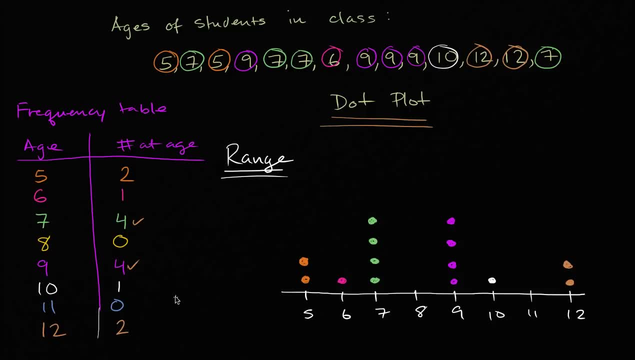 What is the range of age? What are the ages in the classroom? And this is once again where maybe the dot plot is the most, it jumps out at you the most, because the range is just the maximum age in your, or the maximum data point minus the minimum data point. 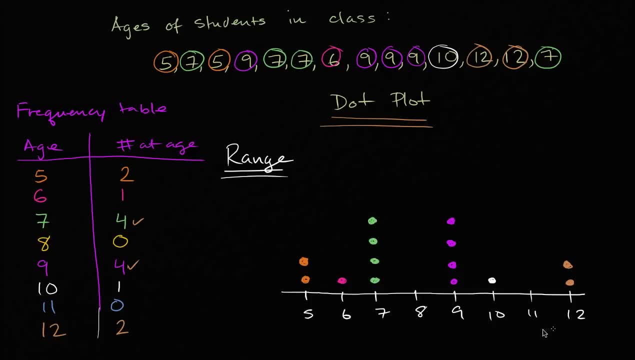 So what's the maximum age here? Well, the maximum age here- we see it from this, from the dot plot, is 12.. And the minimum age here you see, is five. So there's a range of seven. The difference between the maximum and the minimum is seven. 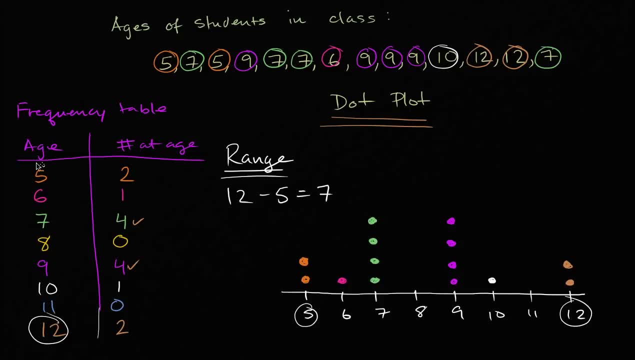 But you could have also done that over here. You could say: hey, the maximum age here is 12.. Minimum age here is five, And so subtract from five, you find the difference between 12 and five, which is seven. Here you still could have done it. 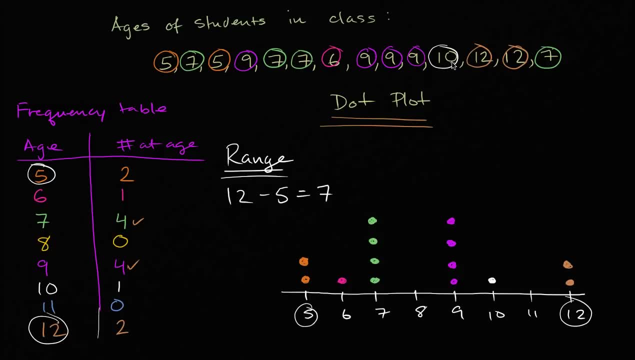 You could say: okay, what's the lowest? Let's look at five. Are there any fours here? Nope, there's no fours. So five's the minimum age. And what's the largest? Is it seven? No, Is it nine? 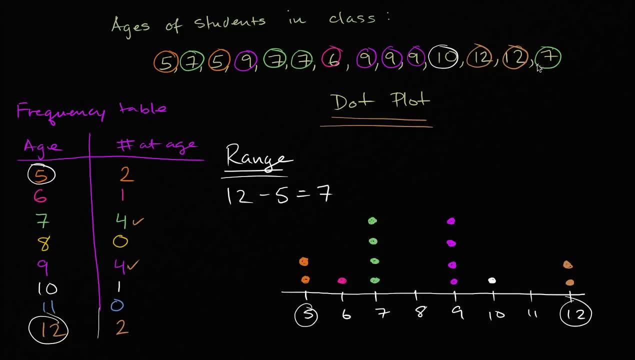 Nine, 10?, Oh, 12, 12.. Are there any 13s? No, 12 is the maximum, So you take 12 minus five is seven to get the range. But then we could ask ourselves other questions.